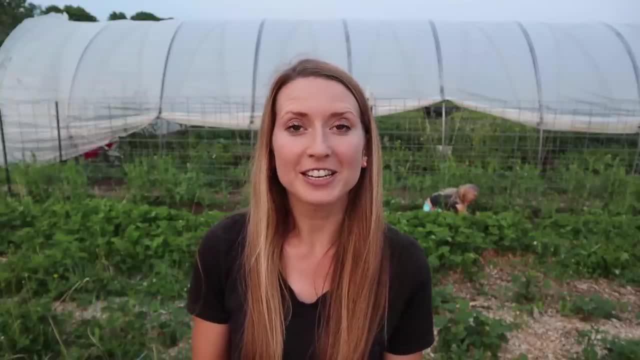 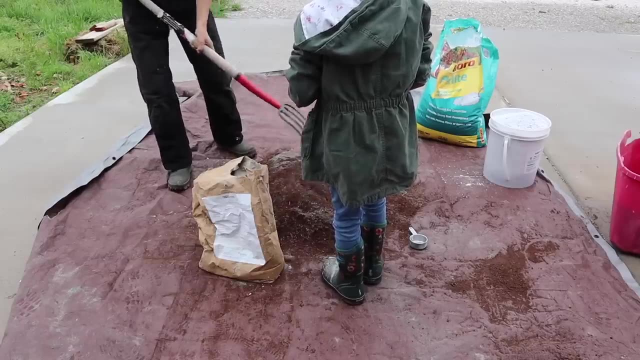 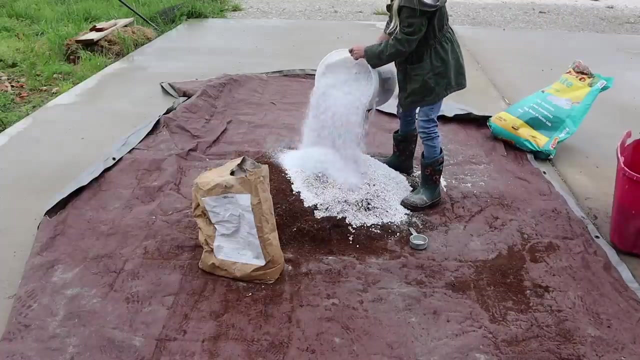 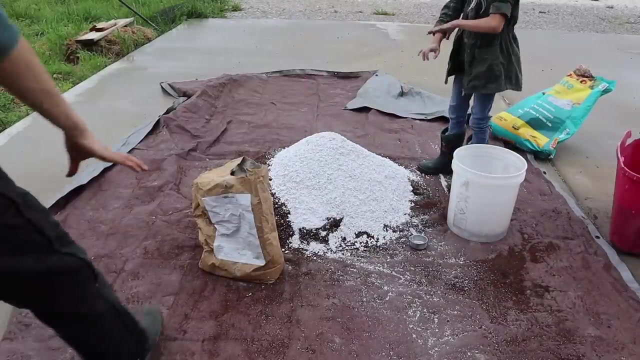 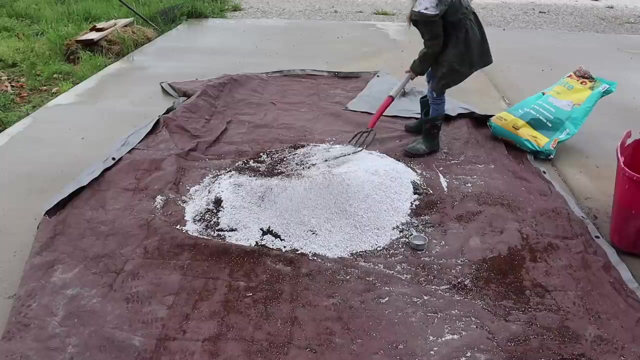 Lisa and Courtney's video down in the video description so you can check them out. That's a lot A double batch, Mom. this is not a very good pitch for it. No, because it kind of goes right through, doesn't it? 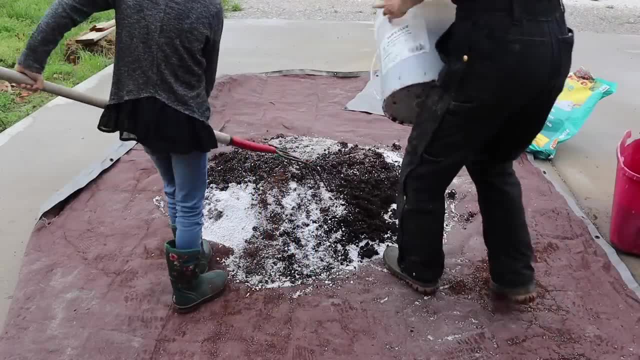 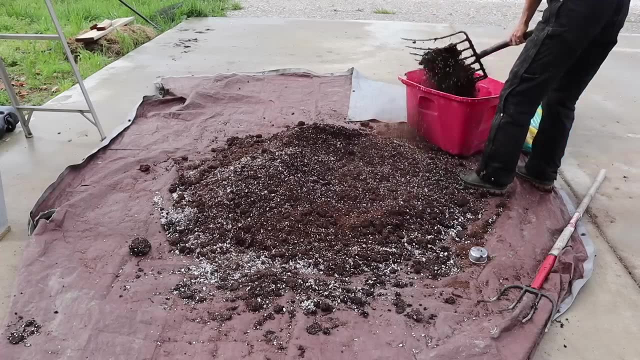 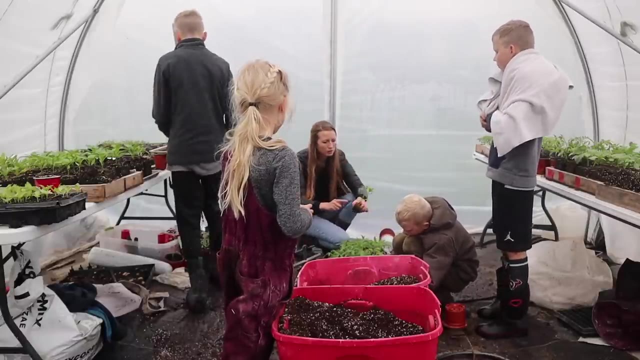 Yeah, More, Yeah, You always have more muscles than girls. You put your, You put your thing on the bottom so that it develops. It'll get all up here, Oh okay. Oh, I just forgot this one. Oh yes. 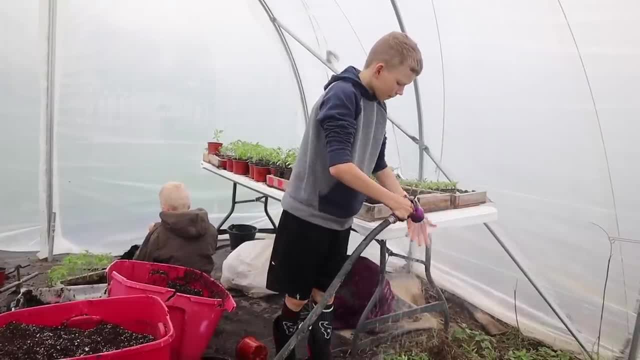 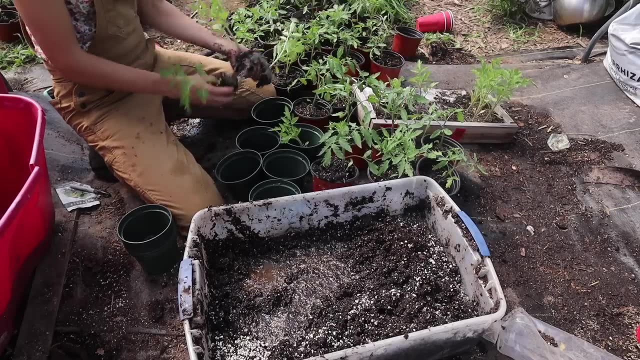 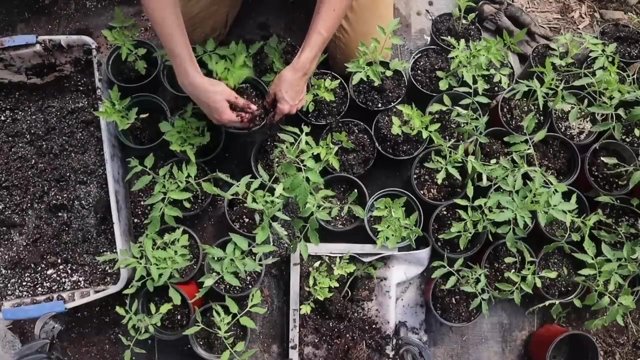 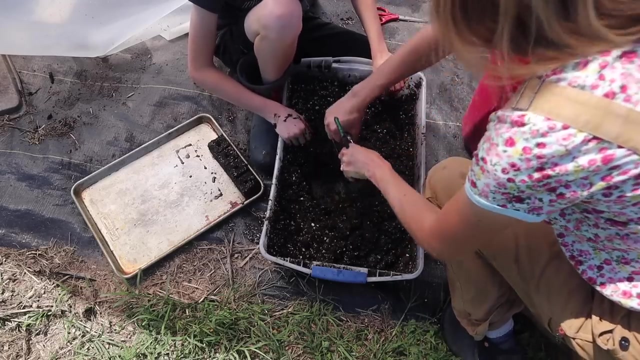 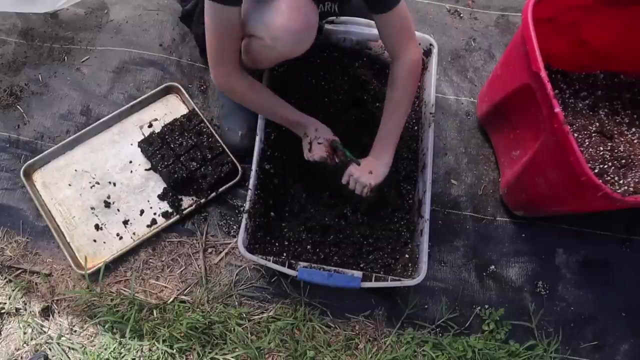 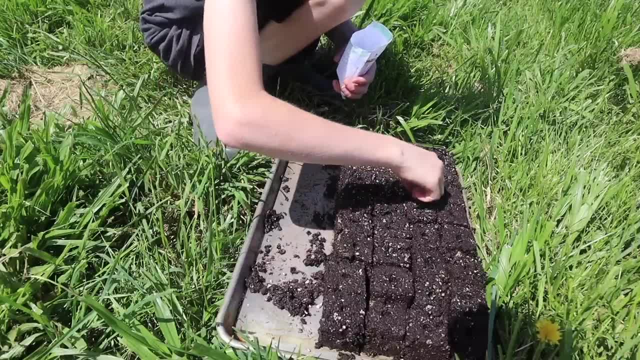 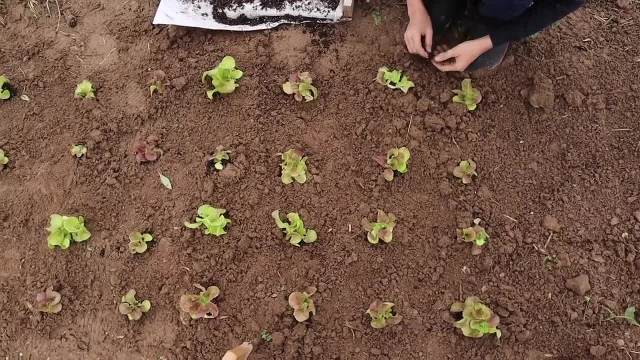 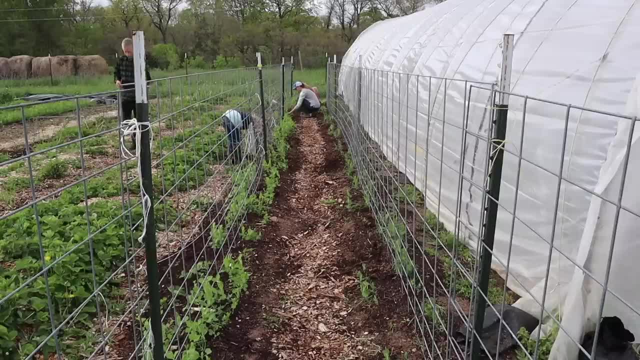 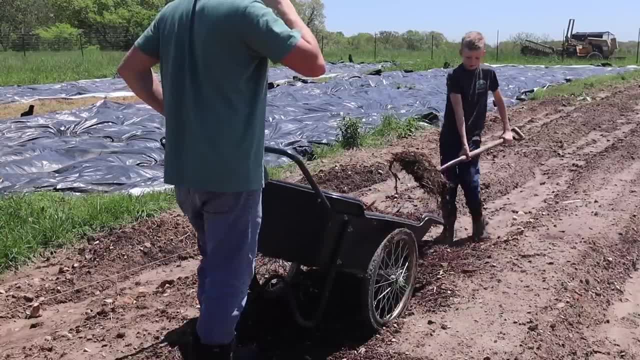 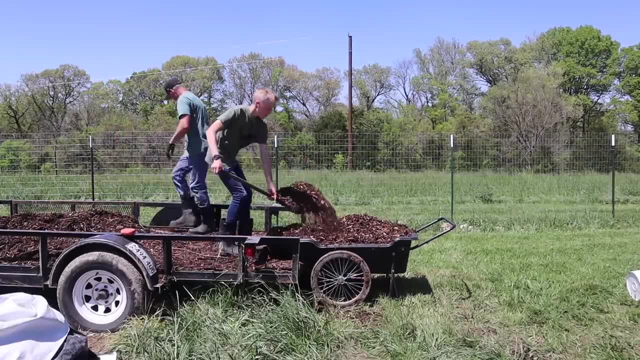 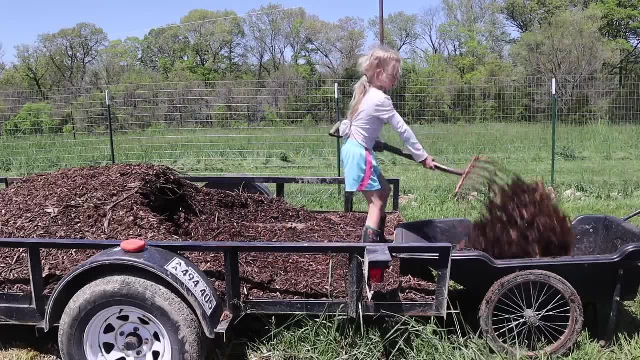 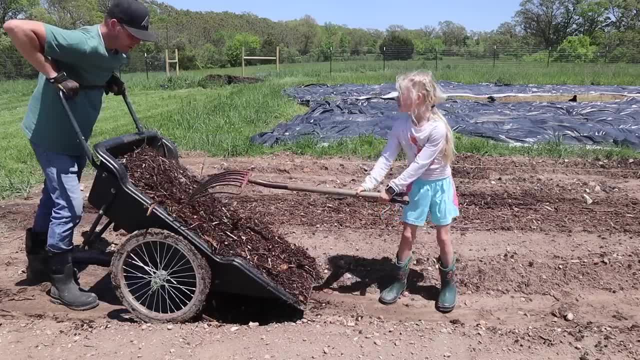 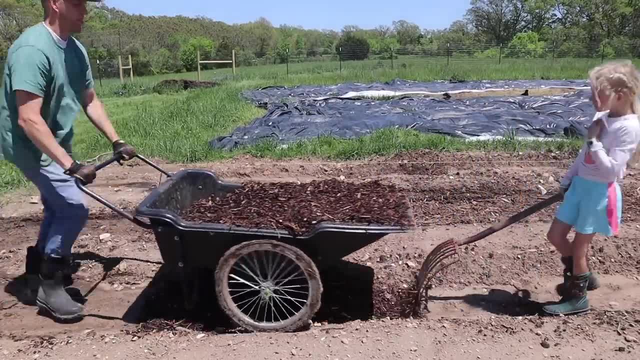 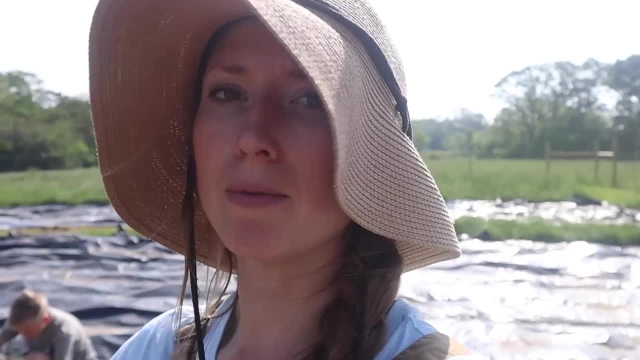 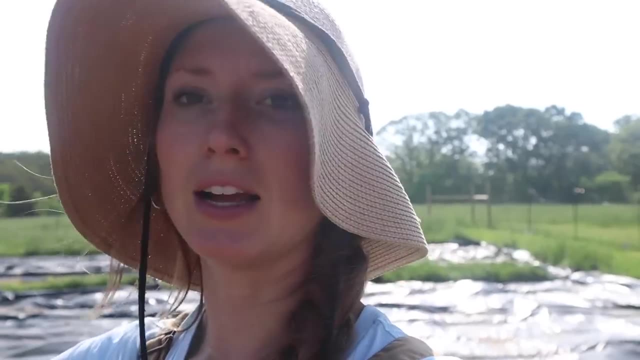 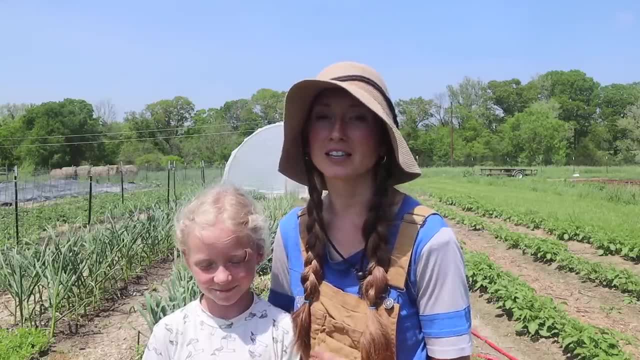 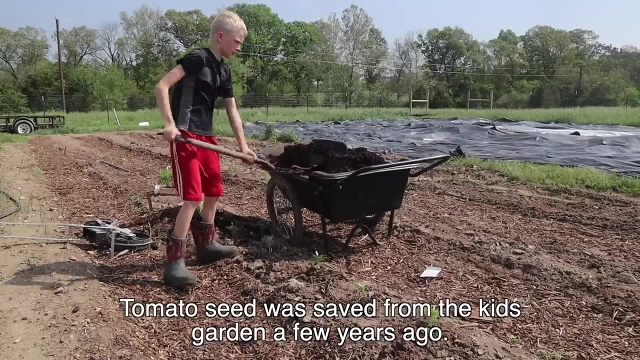 Ever since we have been up here, the kids have not done their own gardens. They've just helped me in the family garden and I knew I wanted to make it a priority this year for them to have their own, because in the past and it's working. 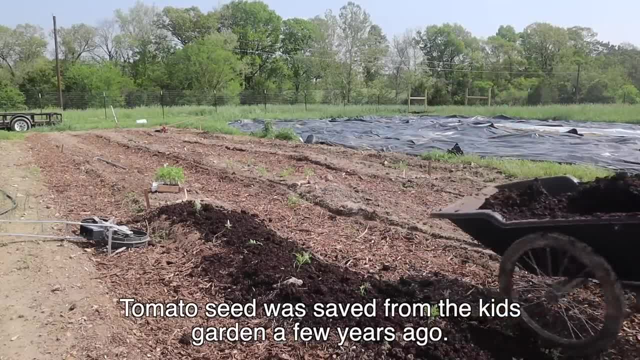 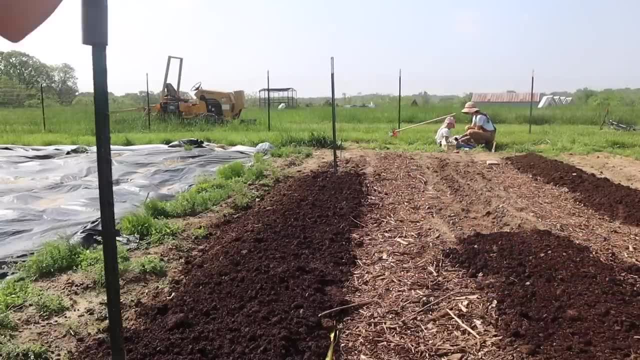 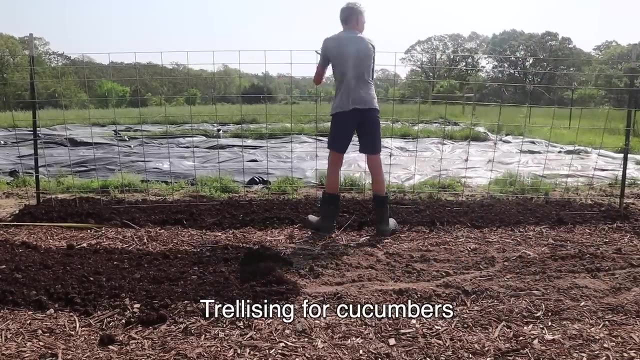 this way, even now, when they have their own gardens, they want to do it and they want to make sure their garden is successful. So they will often go out and weed and water and harvest without any nagging from me or anybody else, which is pretty much the best thing ever. 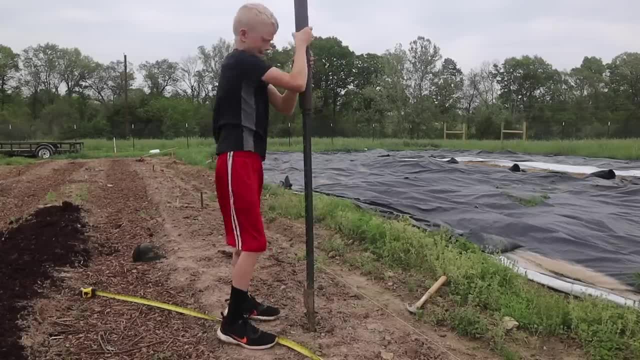 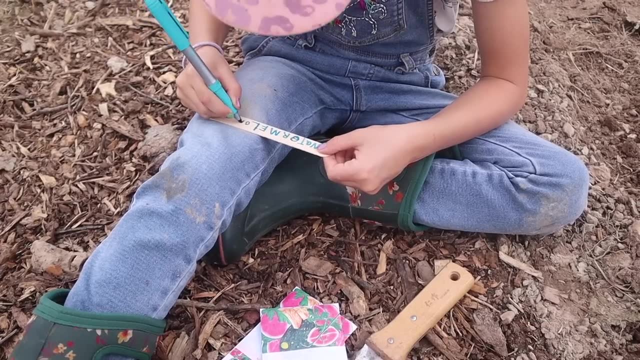 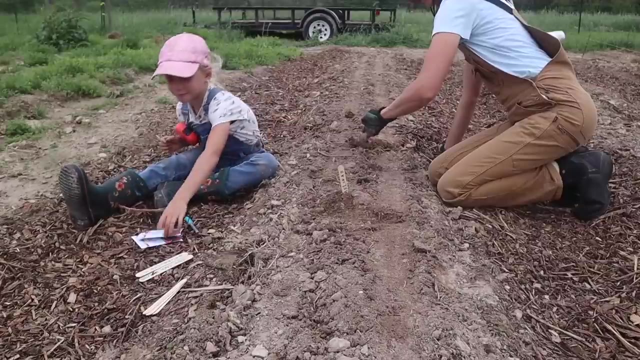 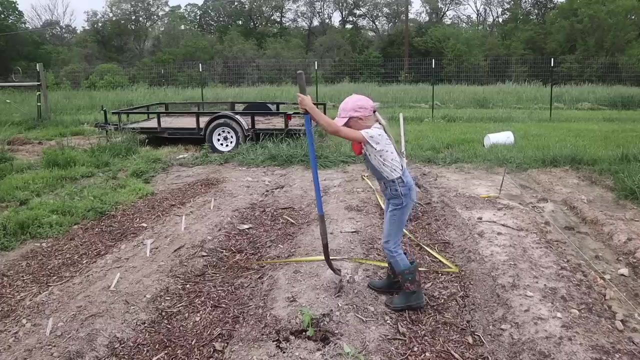 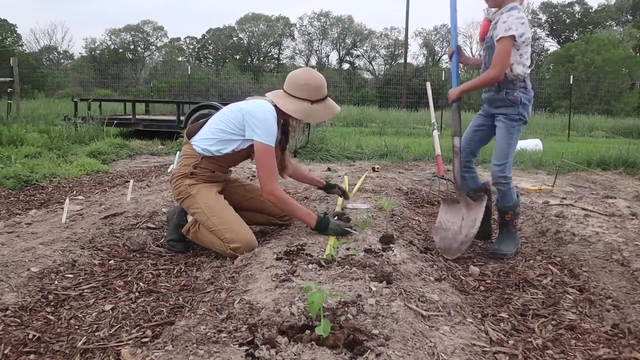 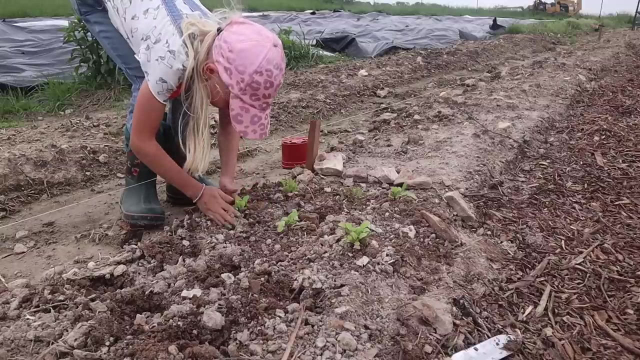 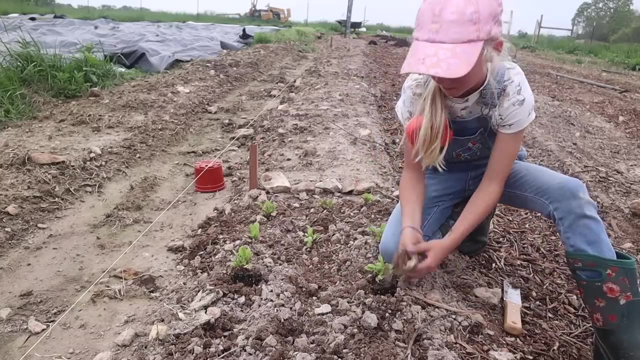 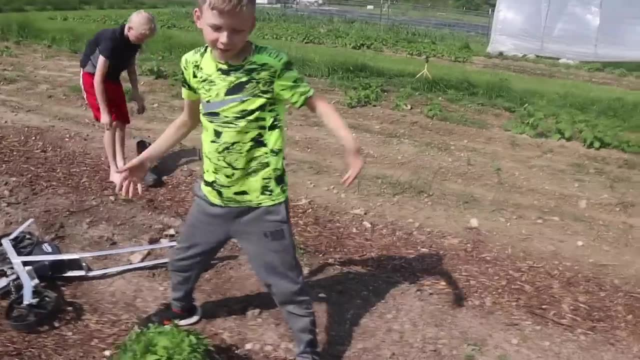 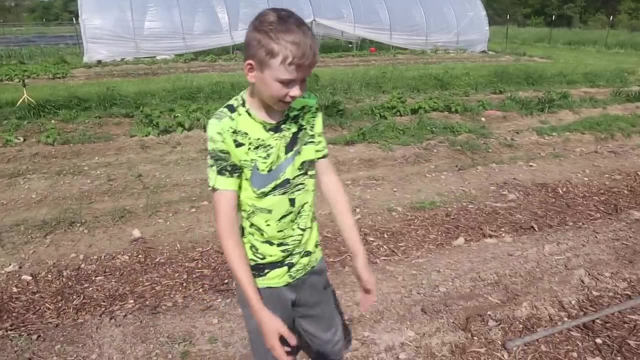 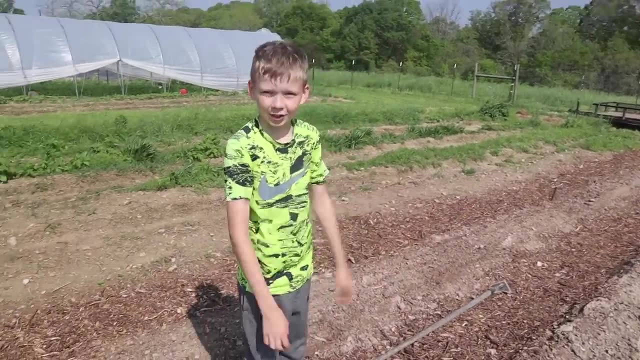 Music. here is the sunrise. bumblebee tomatoes- they are yellow. well, the tomatoes are, but they're not yet. and next is the loofahs. they sprout and then you pick them- they're like over large cucumbers- and you dry them and they're like sponges. how do you like your garden cruise? 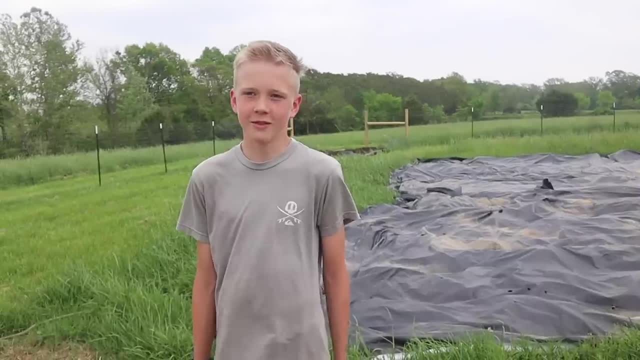 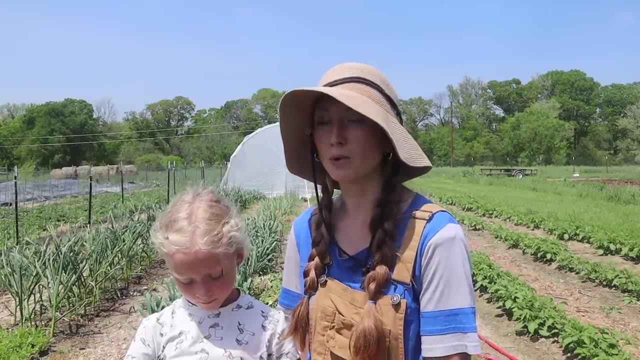 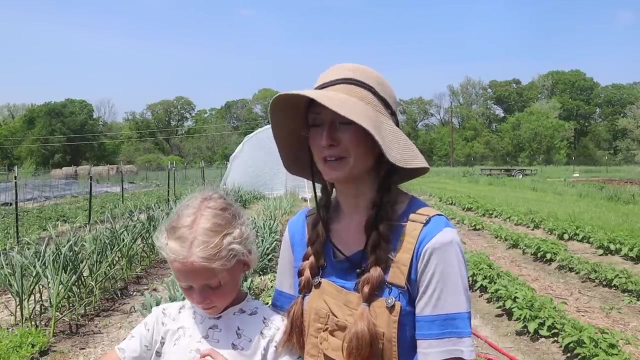 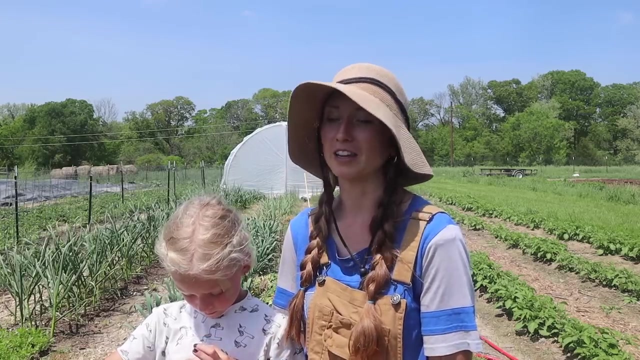 it's best garden i've ever seen. yeah, the funnest time i've ever had in the garden. it was good. they literally spent four or five hours in the garden, but they said that was the most fun i've ever had doing a garden tour because it was their own garden and they could have the creativity to be able to do their own thing. 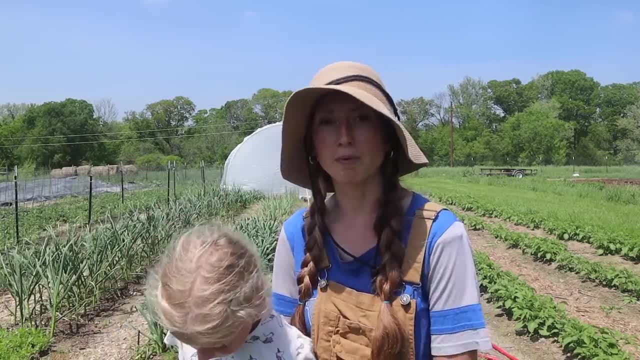 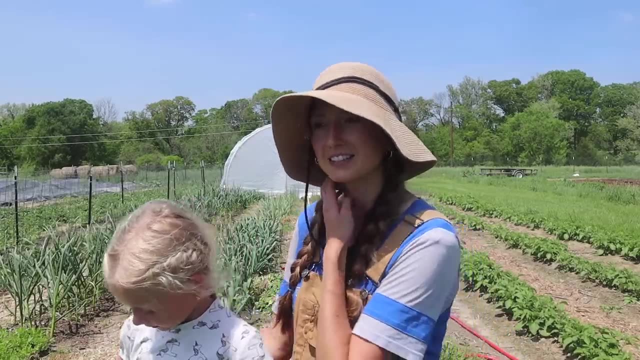 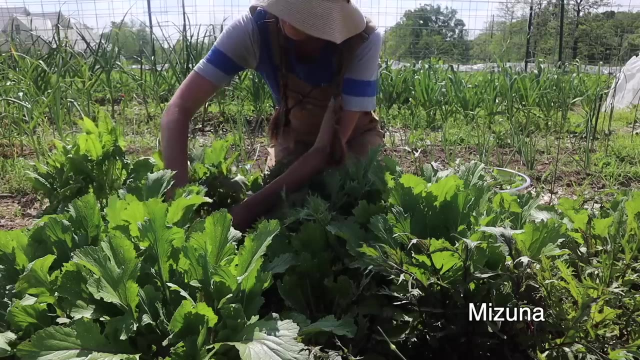 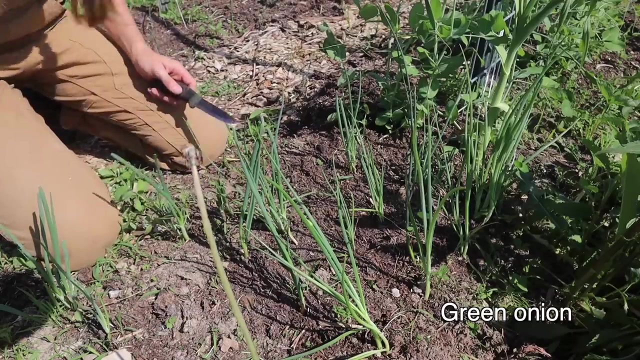 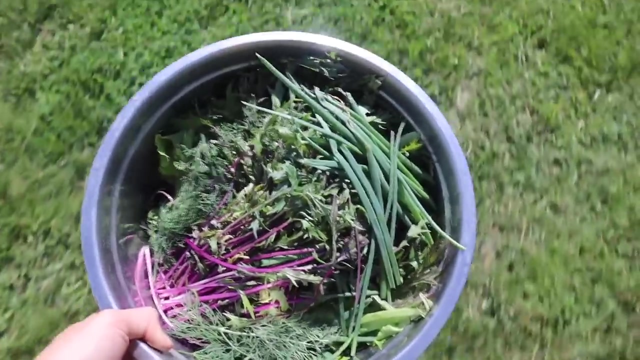 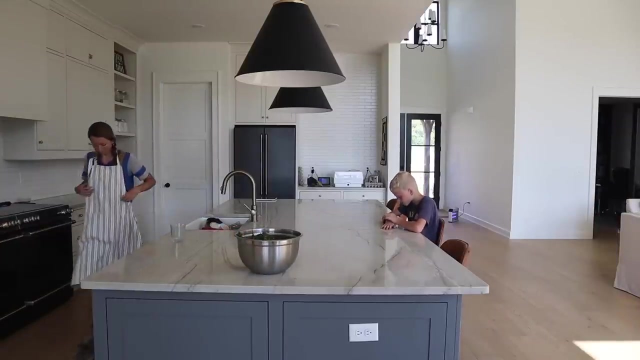 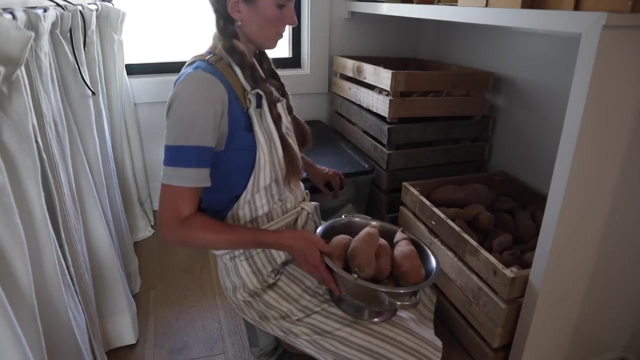 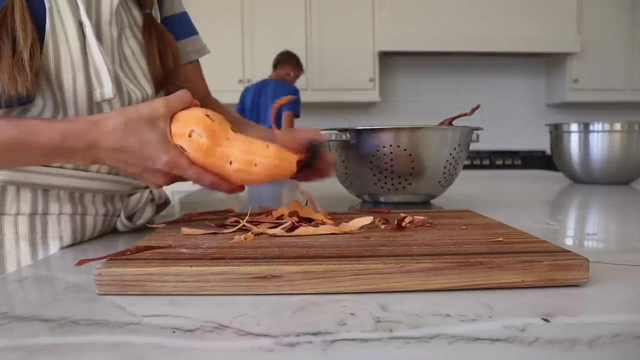 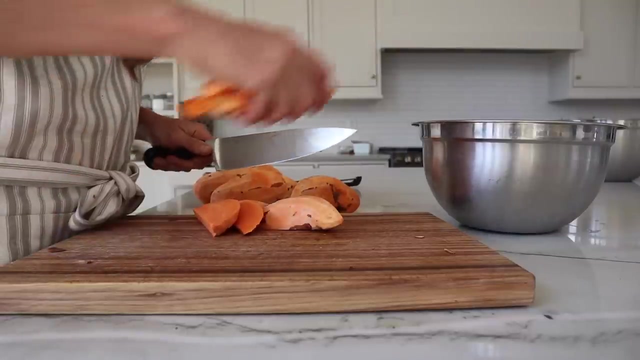 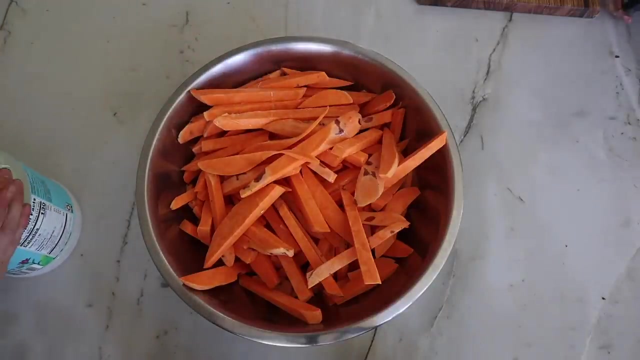 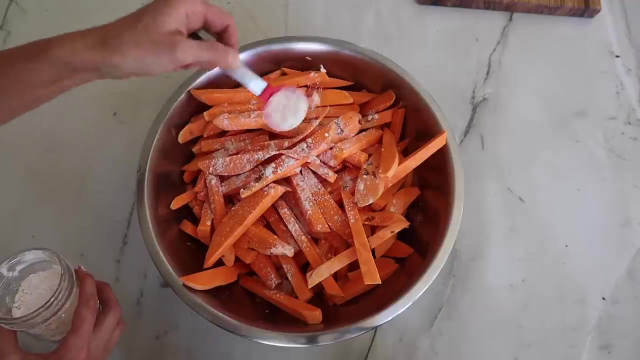 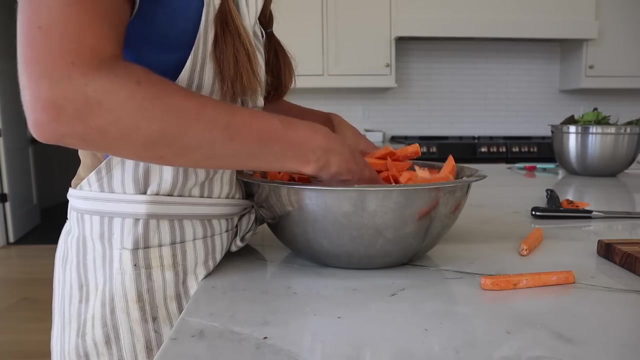 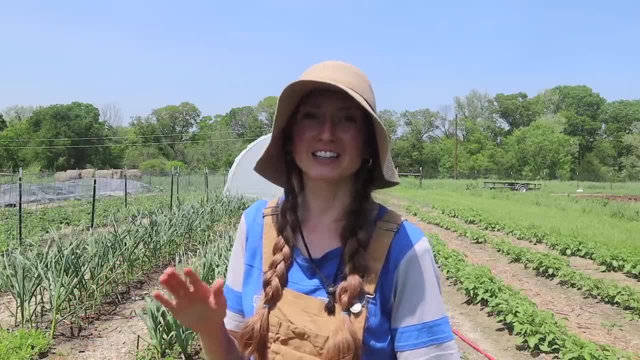 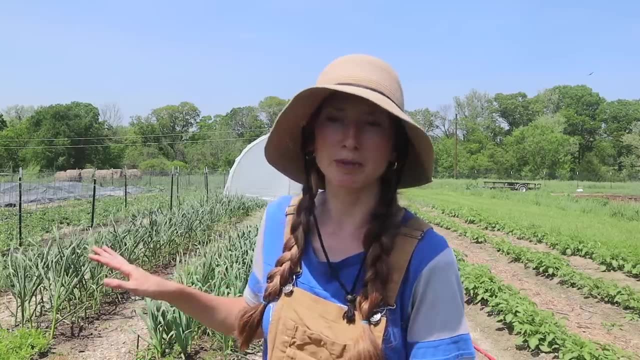 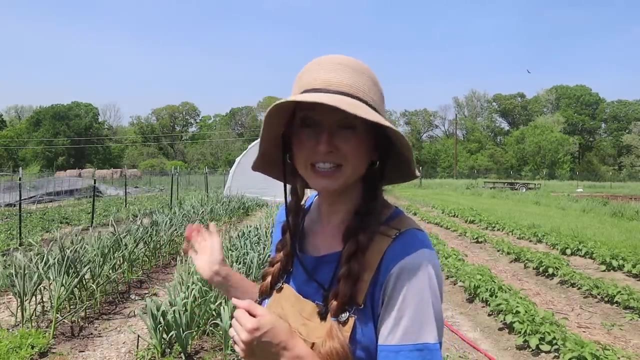 while i was inside cleaning up our lunch, i had a couple of the kids come out and pull out the rest of our spinach crop. it was all going to seed because it's been 90 degrees the past couple of days, so i just had them pull it off and they did a great job. there's still kale in this row which i 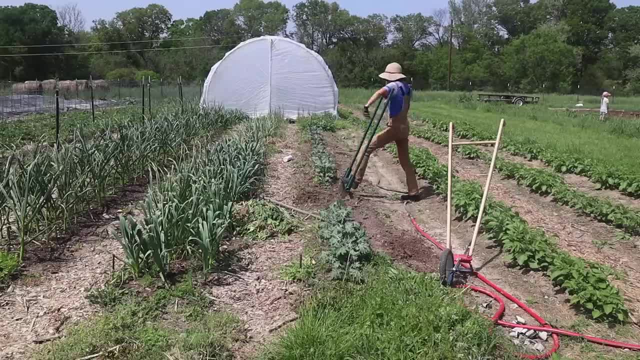 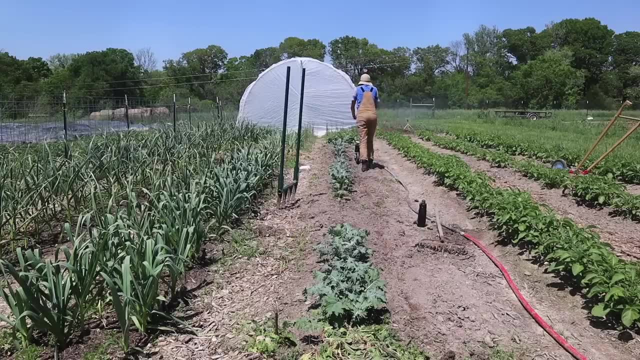 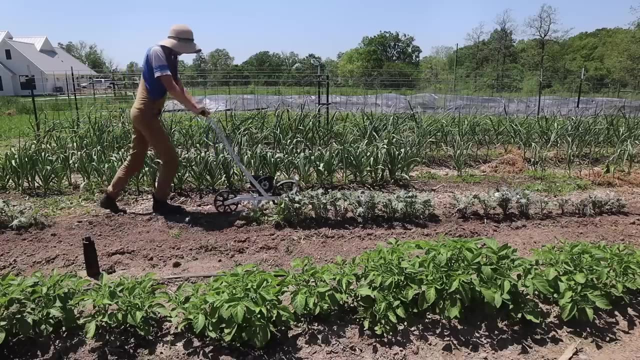 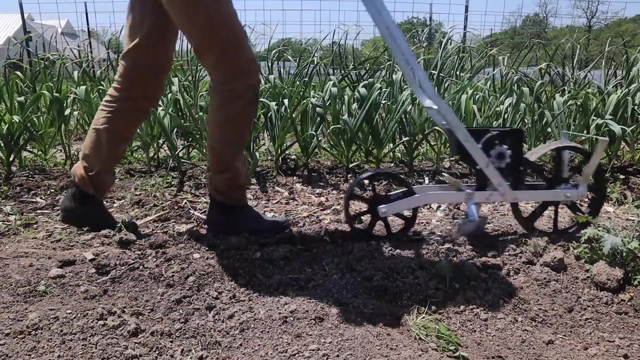 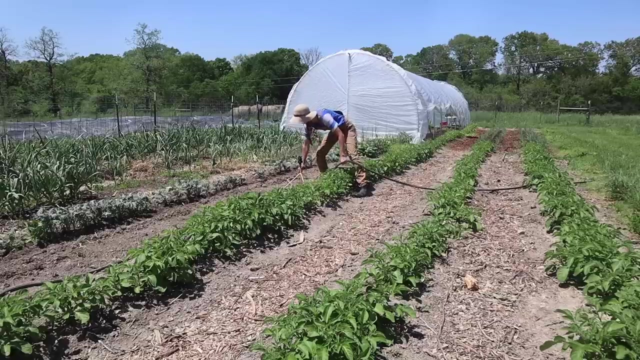 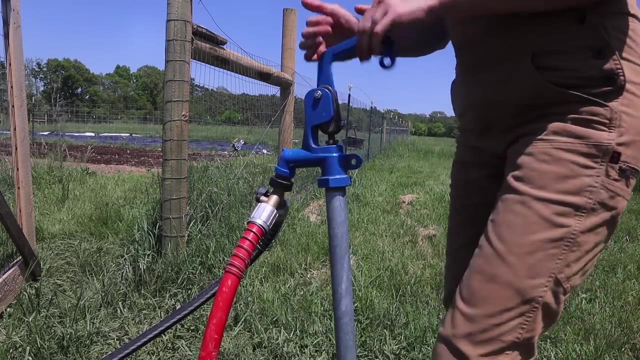 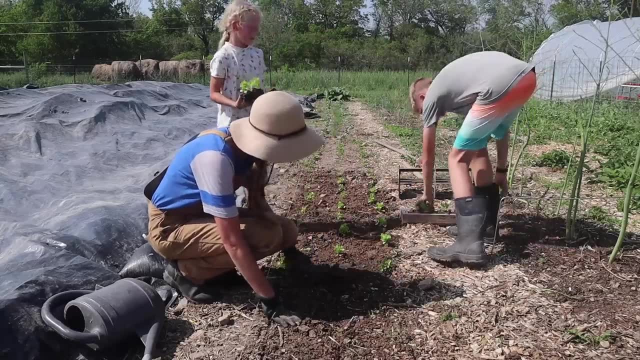 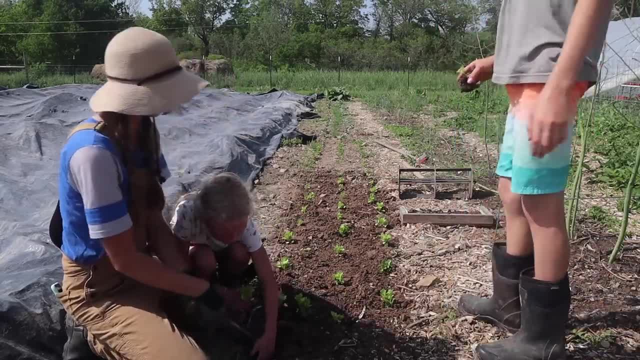 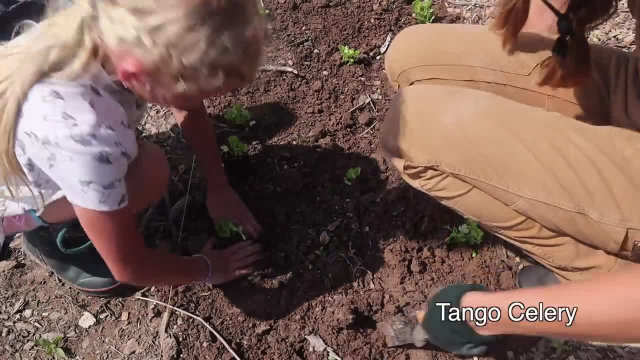 had them leave because it's still good. i'm going to finish cleaning up the rest of that area and then i'm going to plant green beans right along sides of both sides of the kale. so the rest of mine. You got your four. There's actually two more. 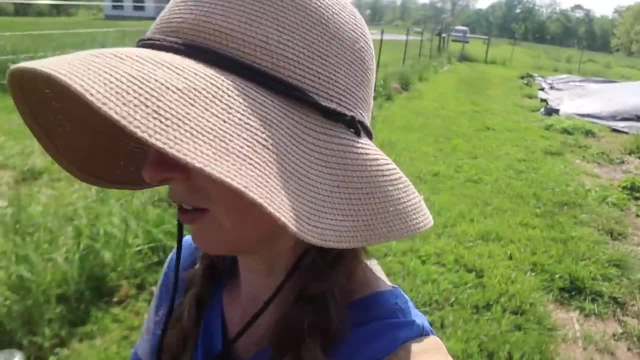 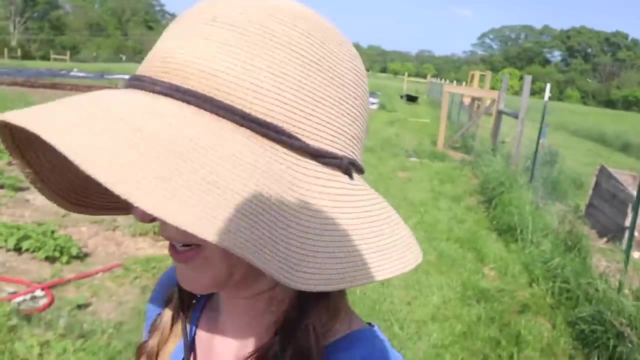 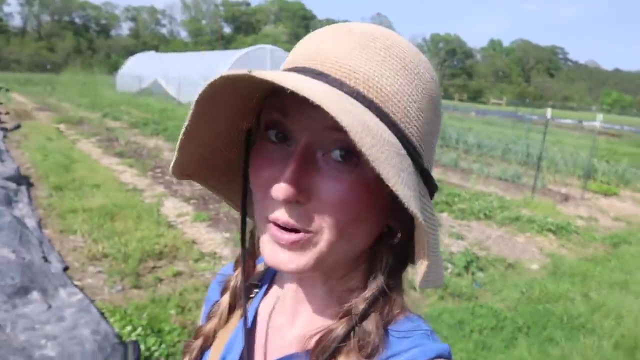 We just finished. We finished planting our celery and the majority of our garden chores are done. It is so hot right now We're going to head down to our creek, take a little break and swim, and then I'm going to come back and weed for another couple of hours. 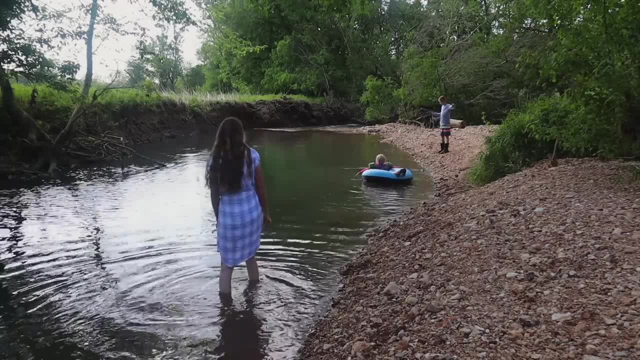 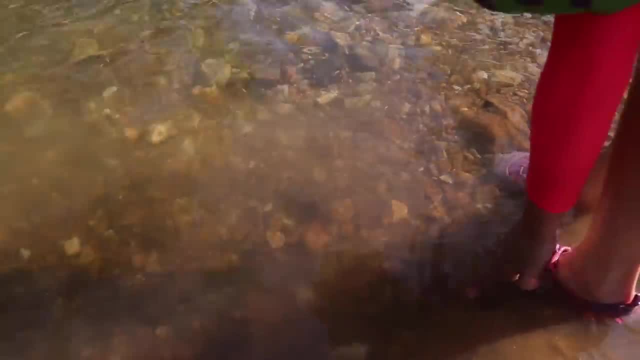 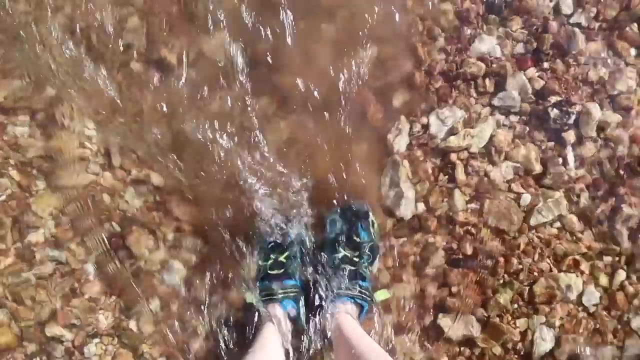 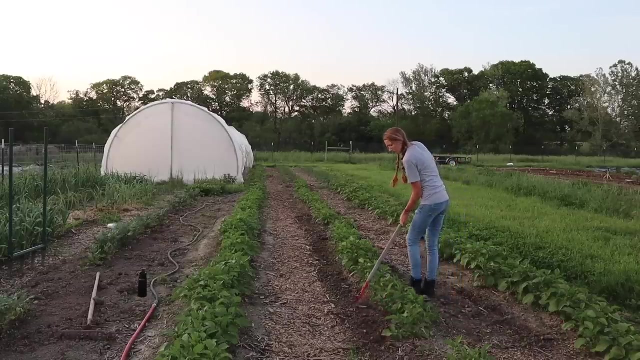 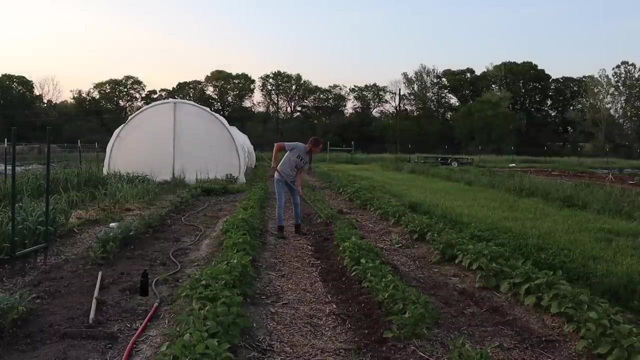 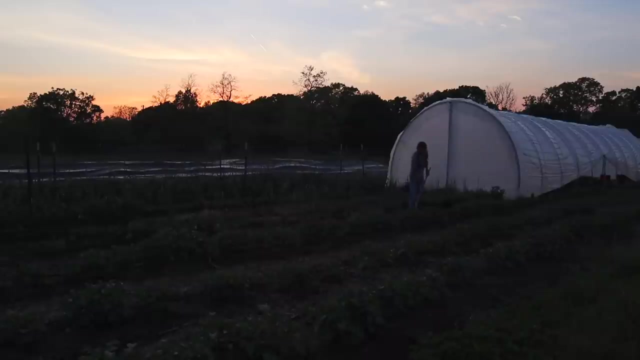 It's so cold. You want to get the crawdad? No, I don't know how to pick him up. Oh, you need your brother, You need your snow. Yeah, That was a good one. It was a great one. 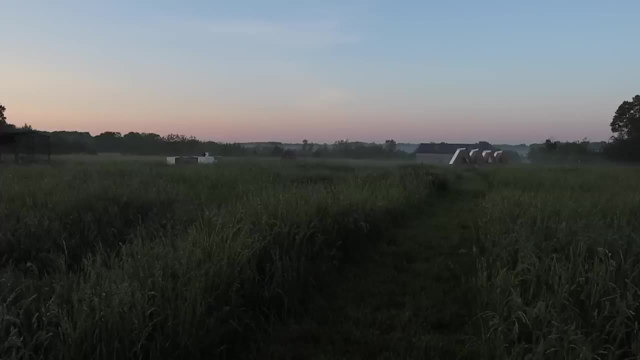 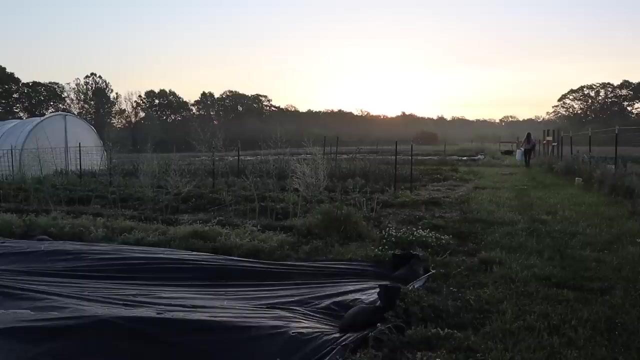 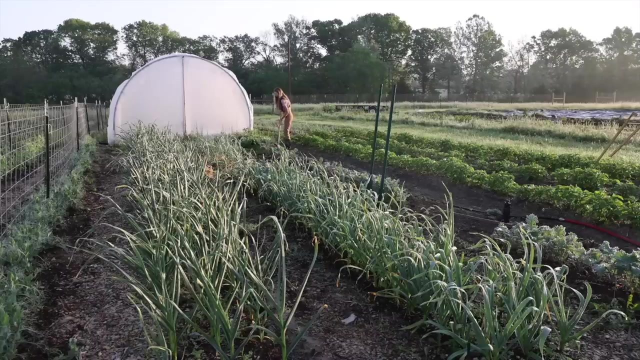 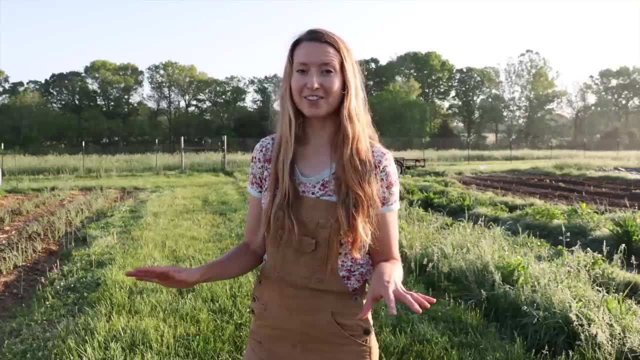 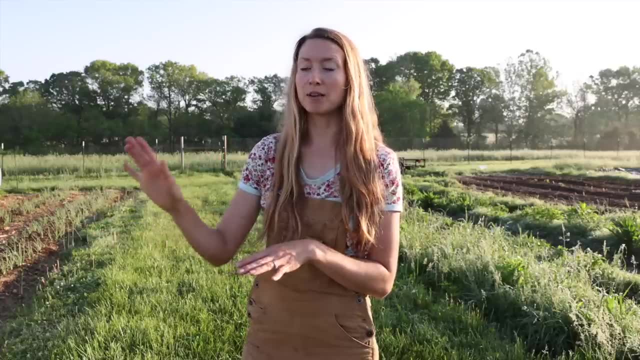 of compost. Some of the kids were able to get compost on their gardens, but some were not and they were not happy about it. And then in the family garden there are areas, like my potatoes, that I wanted to cover with compost and I haven't been. 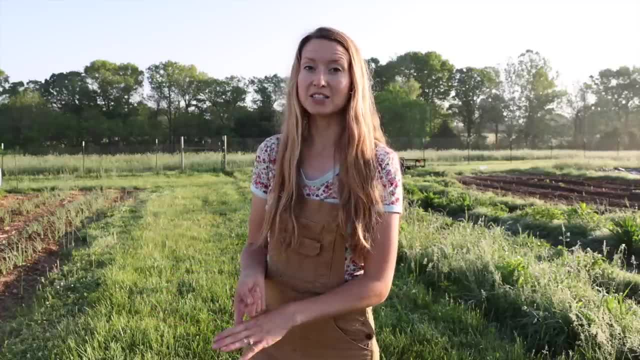 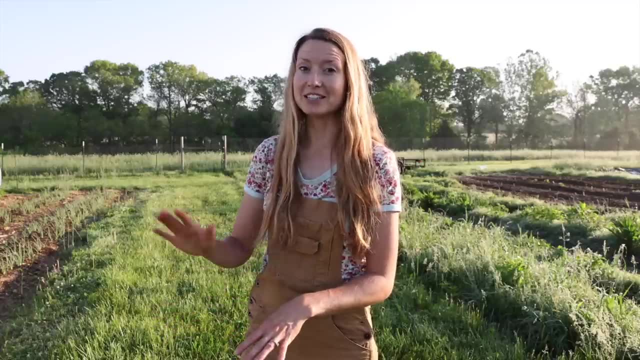 able to do that yet. So Cam is gonna take off of work in a couple of days to go and pick some up because I can't make it fast enough to keep up with the size garden that I have, And the reason he's taking off of work to go and get it is 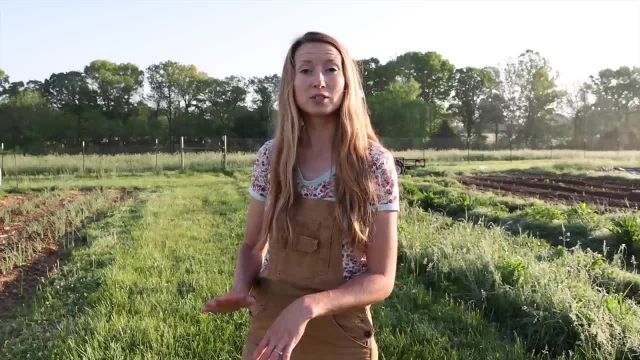 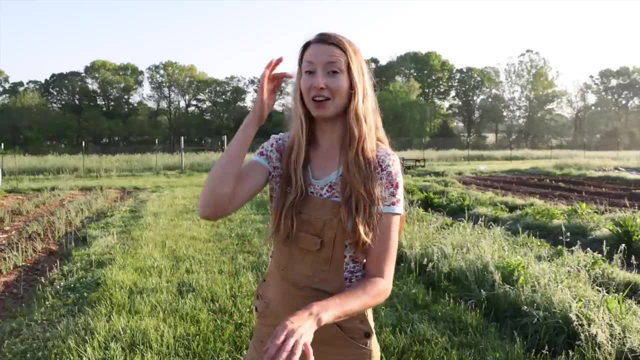 because the place that we really like that has really quality compost is an hour and a half away. We're also renting a trailer to go and pick it up. It may seem like a lot of work, but compost- when you get the right compost, it can really 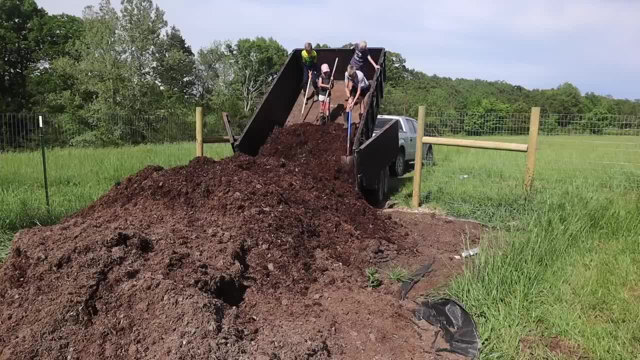 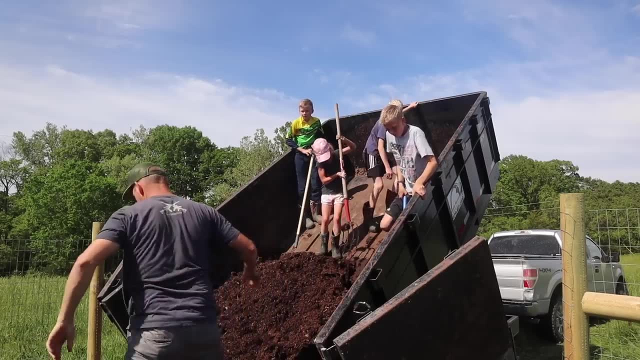 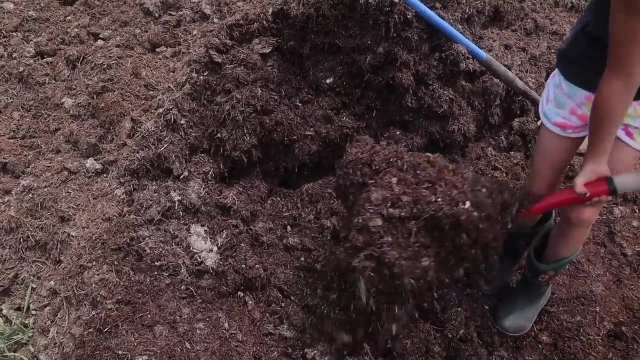 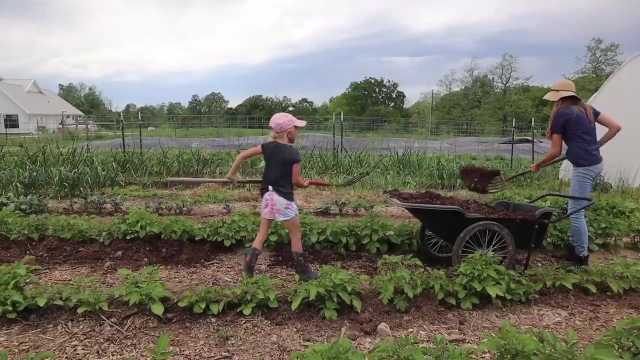 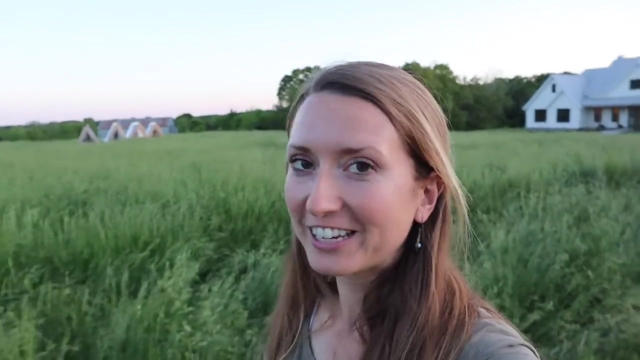 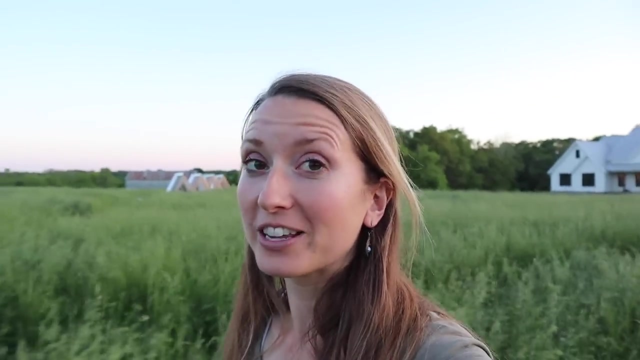 make the difference in your garden So excited that we finally have compost Makes such a huge difference in the garden and keeping the weeds down. and the kids are really excited too. They are gonna put some on their gardens ASAP And then that's really the last step for 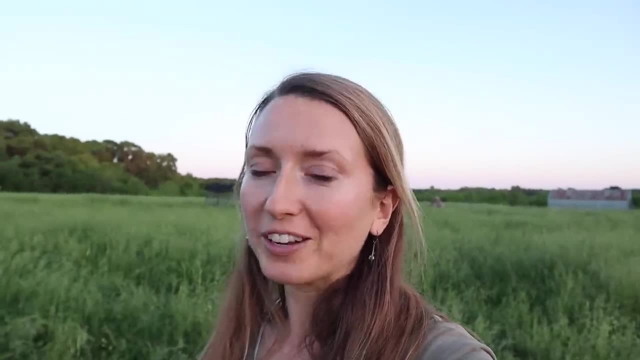 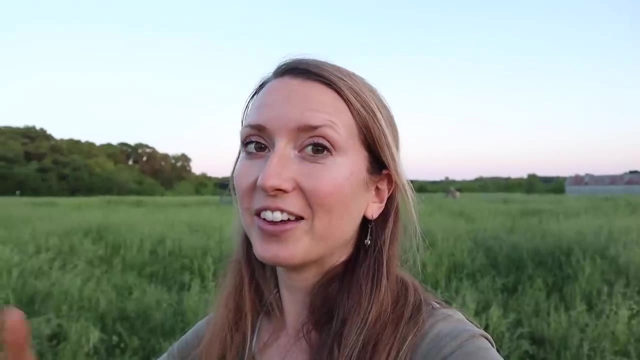 them. They just get to watch it grow. They'll get out there and weed and water. as I already mentioned, they like to do that when it's their own garden, which is just amazing. their gardens give them a lot of purpose and fulfillment. they planted a lot of the summer things like tomatoes and cucumbers. 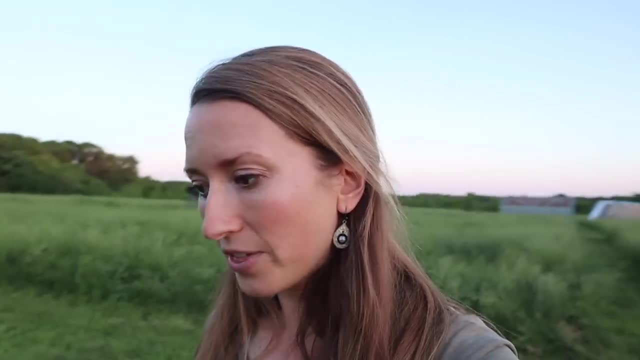 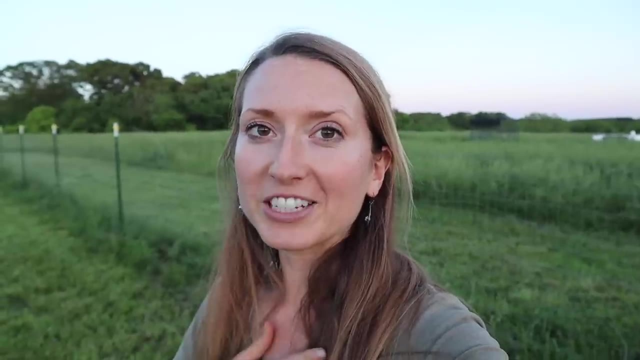 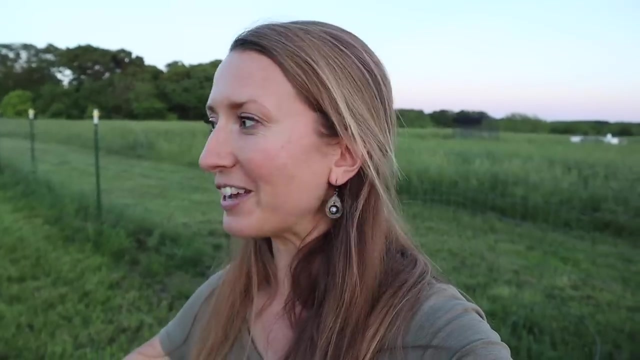 watermelon and corn. so after this initial planting that's pretty much going to be it for the year. they may plant a couple things in the fall. hopefully, when i share the family garden tour, the kids can share maybe some of their gardens at the end of that tour as well, so we can keep. 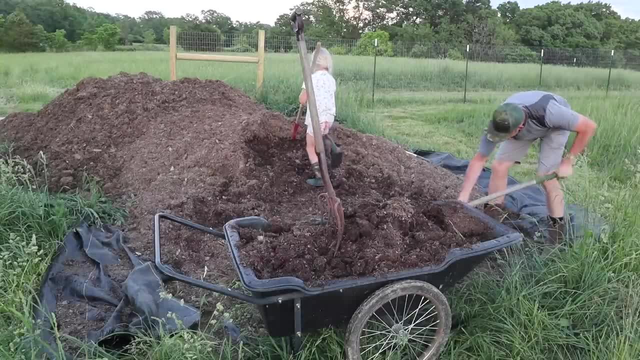 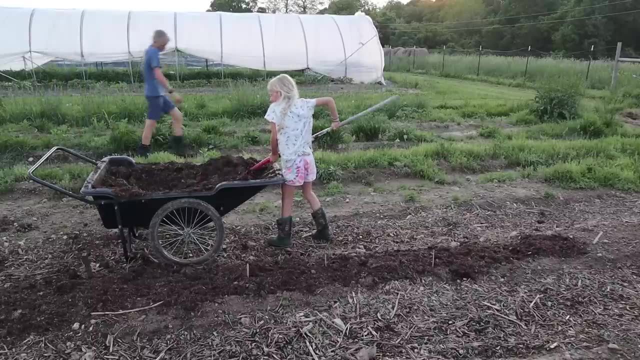 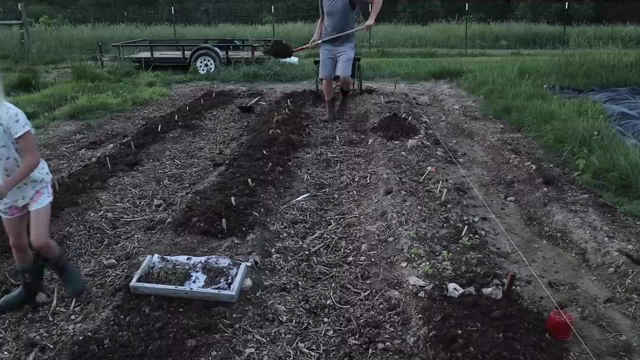 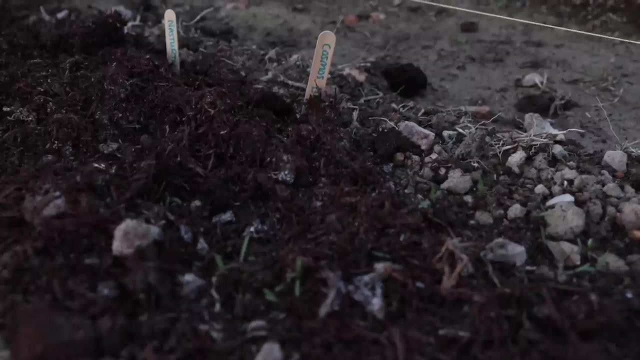 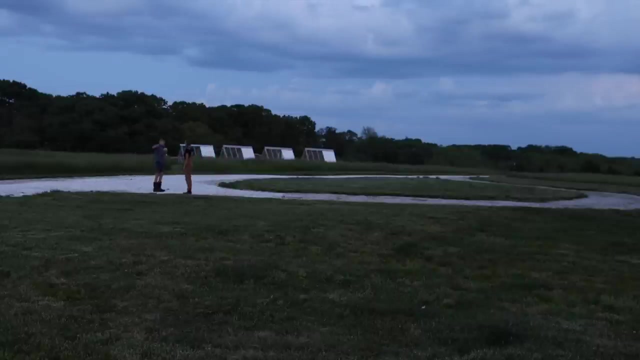 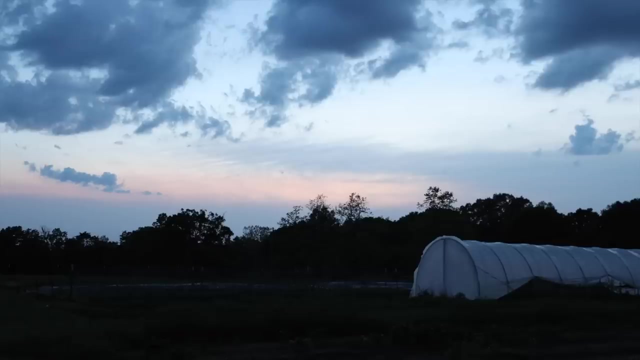 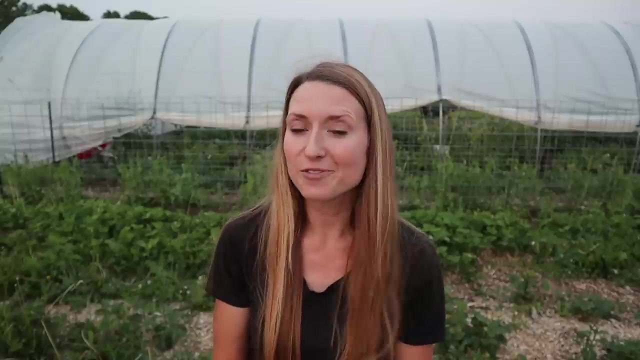 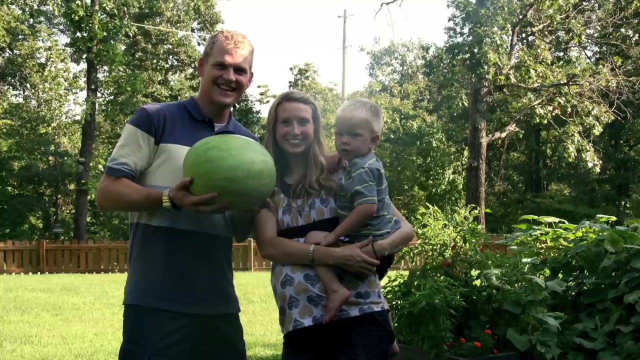 you guys updated on how it looks and each different garden. it's been so fun to see how their personalities come through each of their gardens. i have been gardening for 15 years and my oldest is 14, so all of my kids have been gardening with me their whole lives and i have learned some things over the years to help to keep them. 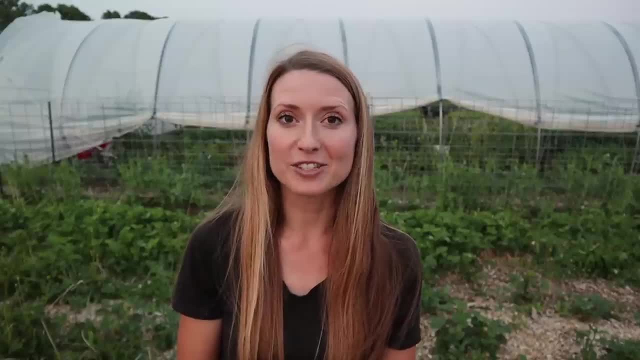 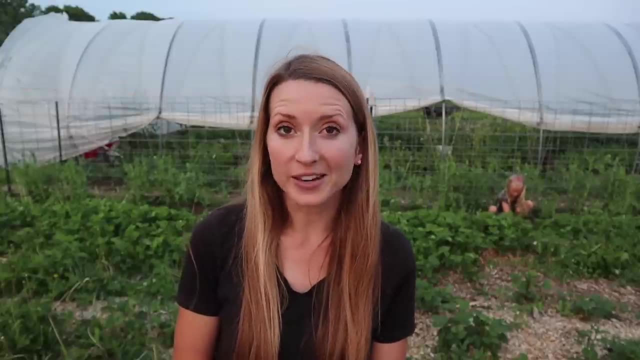